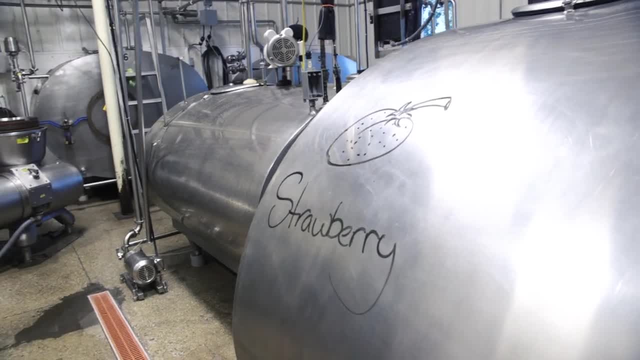 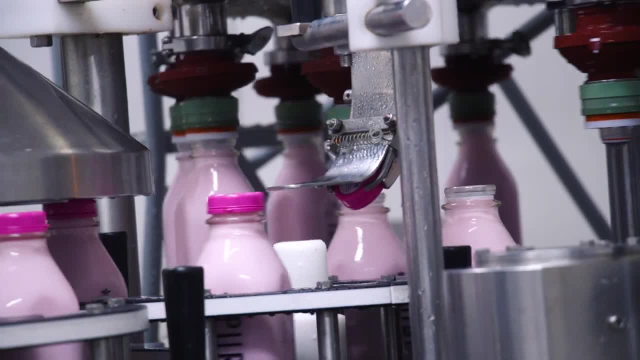 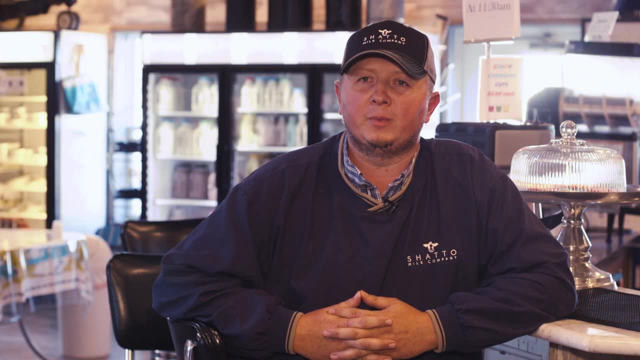 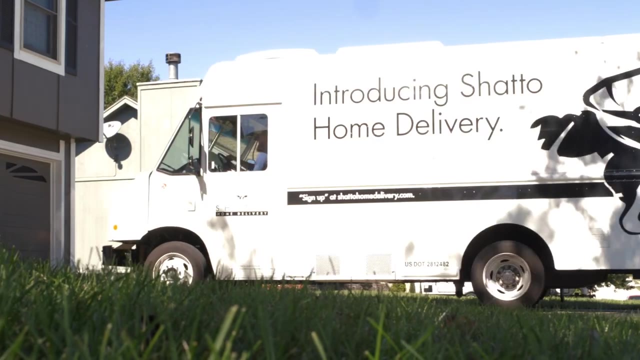 By us doing something different with the glass bottles. I think that brought in a whole new perspective of you know, let's bring back the milkman that brings our milk right to the door. A lot of generations have not seen that. I think the trend of you know, everybody delivering to 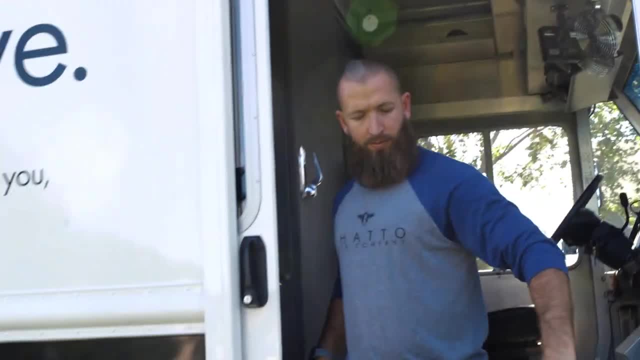 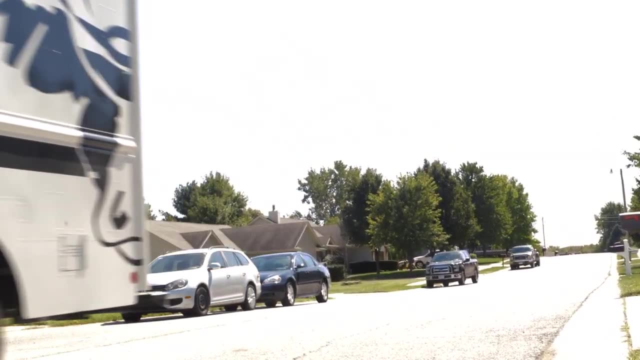 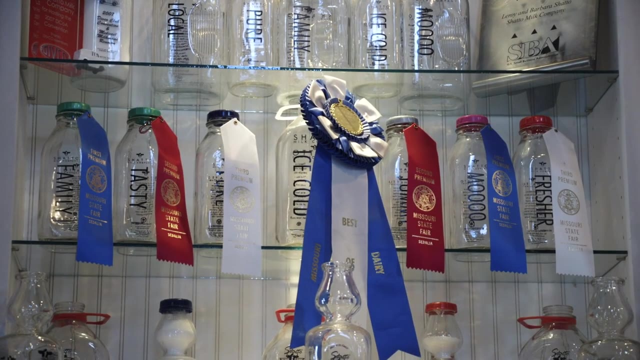 everybody's doorstep continues. You know, we're just kind of the leading edge of of an old technology. I think We've competed a lot in the world dairy products and won several awards with our root beer milk, some of them with our butter. 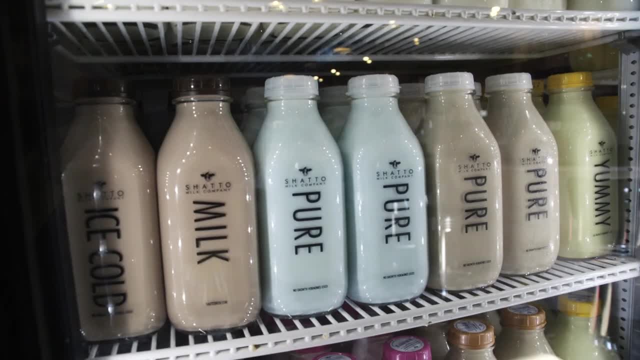 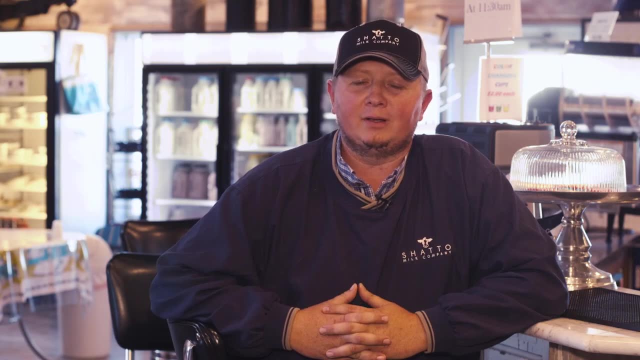 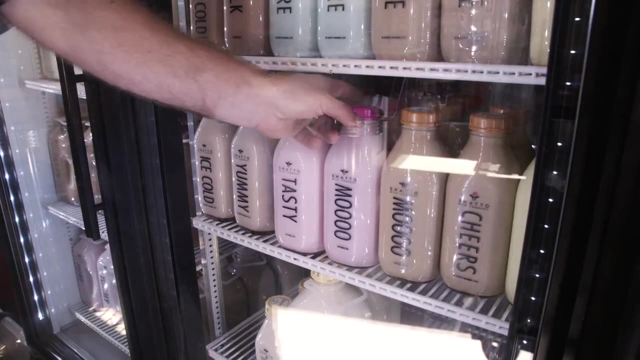 some with our chocolate milk. The chocolate milks also traveled to the White House Dairy farming. you put a lot of hours in, you put a lot of time and effort into things and just to have that product going out to consumers and feeling confident that all that hard work. 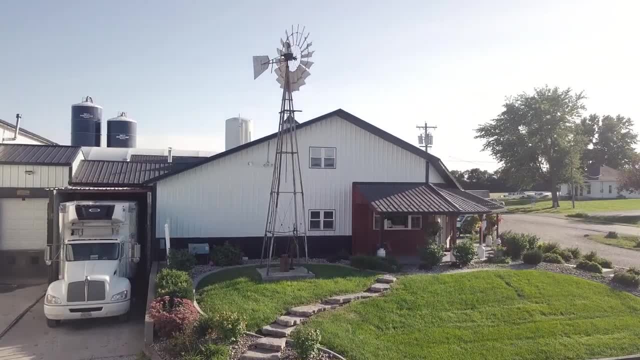 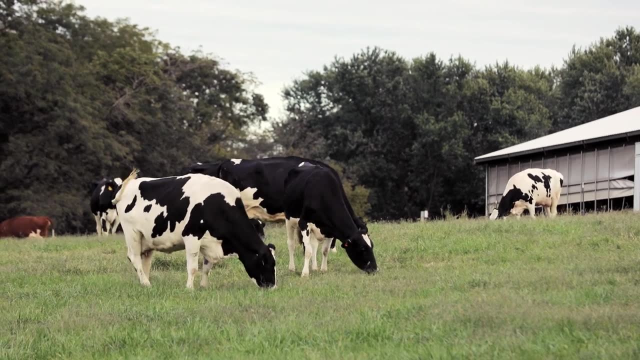 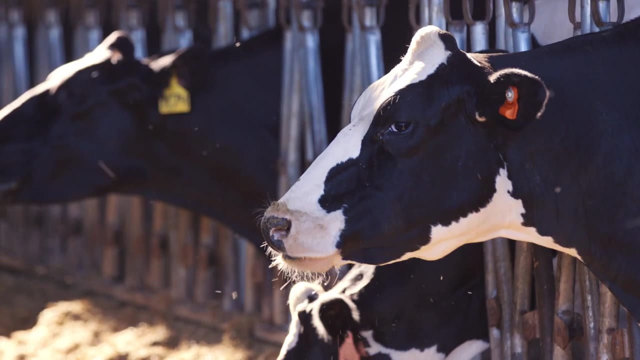 you've done a good job. you're putting a product out there that's a healthy, wholesome product. The Holstein cow has been an icon in all of agriculture for many years and I think it kind of gives you a sense of pride. It's the perfect cow for what we're doing here. 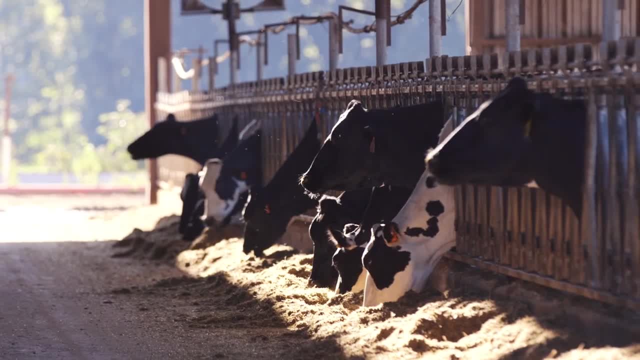 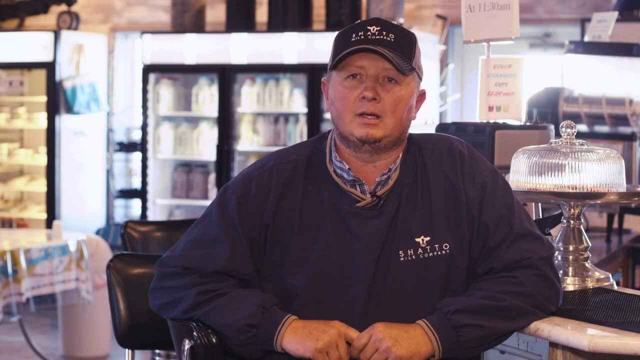 with all the information we can gain. We've been registering cows here for about five years. We've started out with a basic ID, registering our grade cows up, and that's been beneficial in selecting new sires and animals that will perform better in this herd. 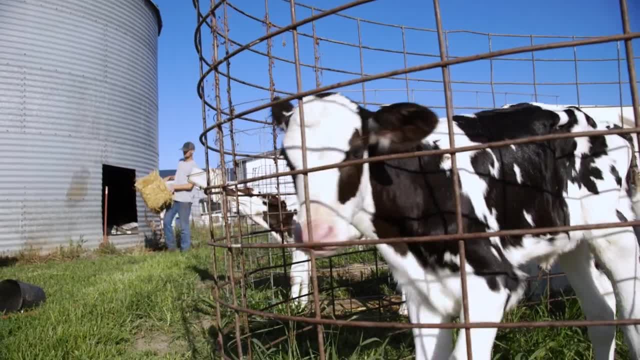 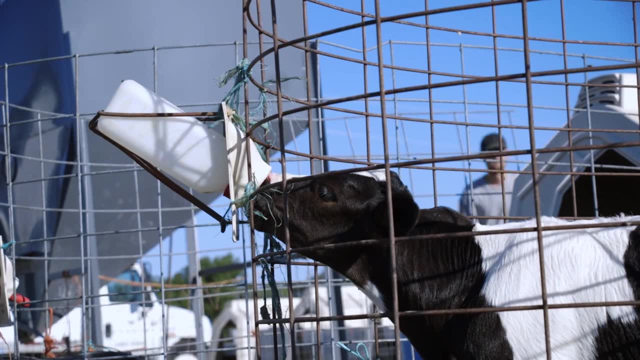 Just allows us to look into the future a little bit farther. It's good to collect all that data so that we can not just two years down the road, but five years or 10 years down the road still be making a better cow. 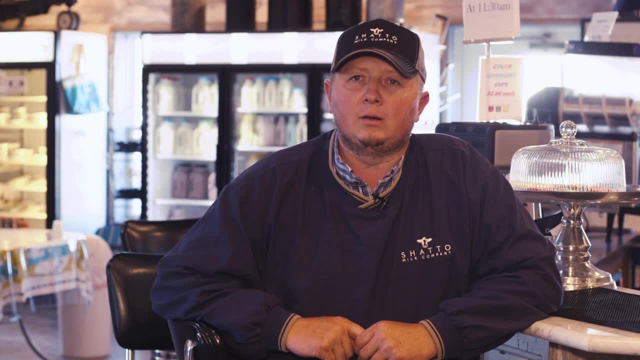 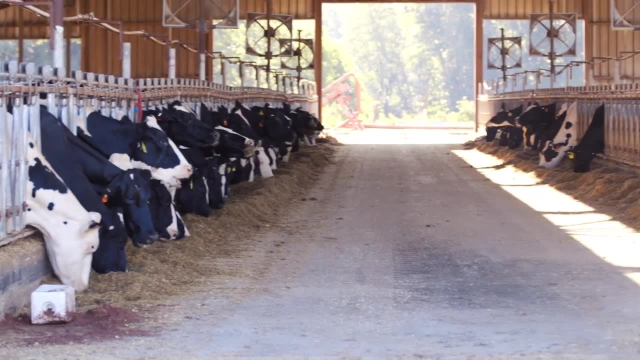 By selecting and moving to the registered side we've been able to reduce the total number of animals here but get higher production out of those cows. We've dropped about 100 animals from when we were doing just grade cows to the registered Holstein cows. 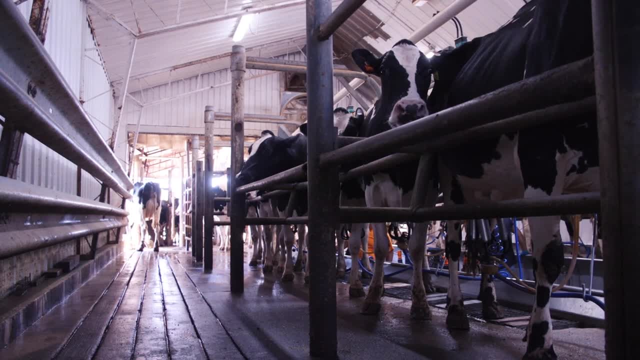 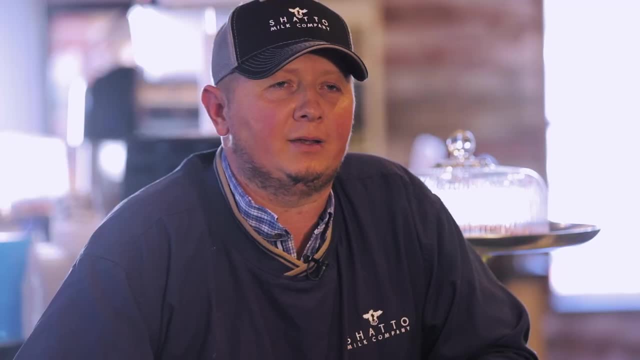 The registered Holstein allows us to do such a variety of things and allows us to put a variety of products out for our customers and, I think, for the future. With all the information we can get, I think the sky's the limit of what we can do.